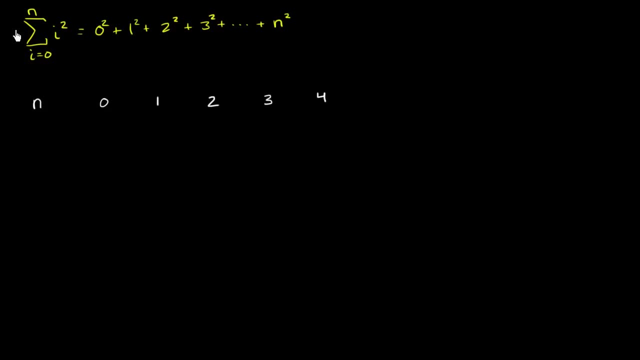 And now, for each of these, let's see what the output of our function should be. The output of the function should be this thing: It should be the sum from i equals 0 to n of i squared. So when n is 0, well, that's just going to be 0 squared. 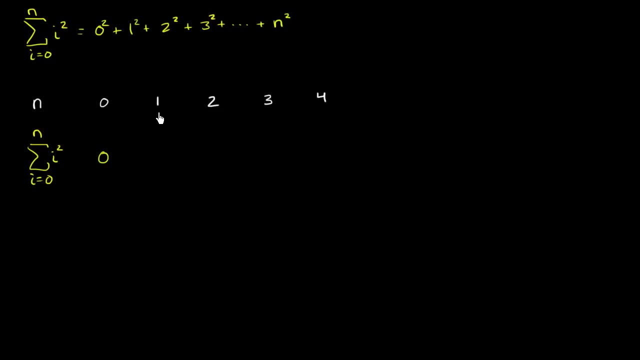 We just stop right over there, So that's just 0.. When n is 1, it's 0 squared plus 1 squared, So that is 1.. When n is 2, it's 0 squared plus 1 squared plus 2 squared. 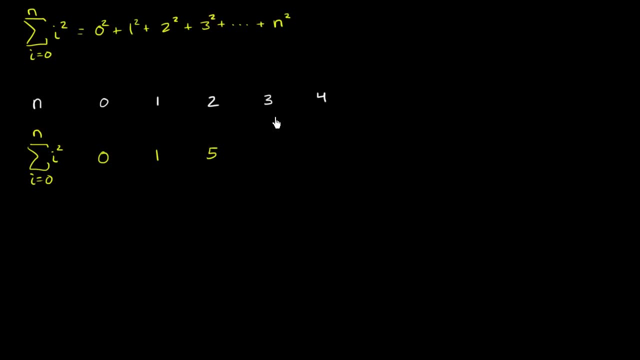 So that's 1 plus 4,, which is 5.. When n is 3,, now we go all the way to 3.. So it's going to be 1 plus 4,, which is 5, plus 9.. 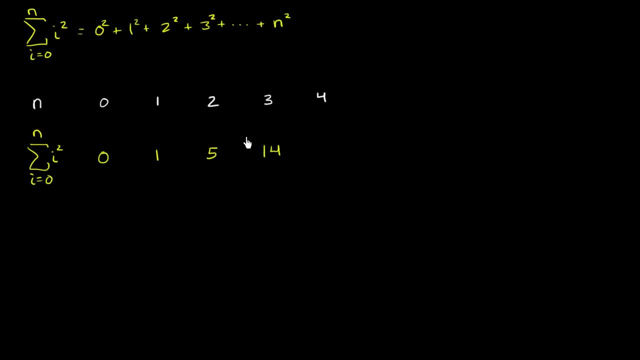 So 5 plus 9 is 14.. And then, when n is 4,, we're going to add the 16, 4 squared to this. So this just gets us to 30.. And of course we could keep going on, and on, and on. 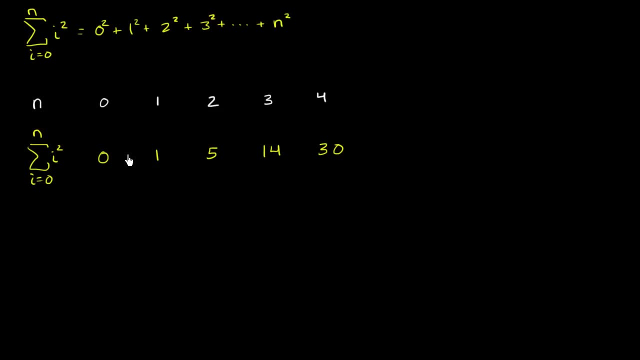 So let's study this a little bit to think about what type of a function for each of these inputs might give us this type of an output. So let's first look at the difference between these terms. So the difference here is 1.. The difference here is 4.. 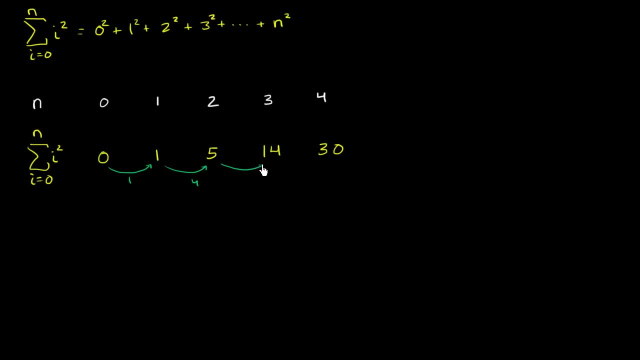 This is obvious. We added 1 here, We added 2 squared here, We added 3 squared or 9 here, We added 4 squared or 16 here. And the reason why I'm doing this is if this was a linear function. 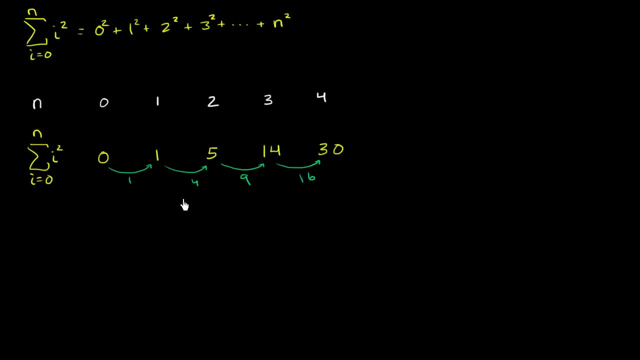 then the difference between successive terms would be the same. Now, if this is a quadratic function, then the differences between the differences would be the same. Let's see if that's the case. So the difference here is 1.. The difference here is 4.. 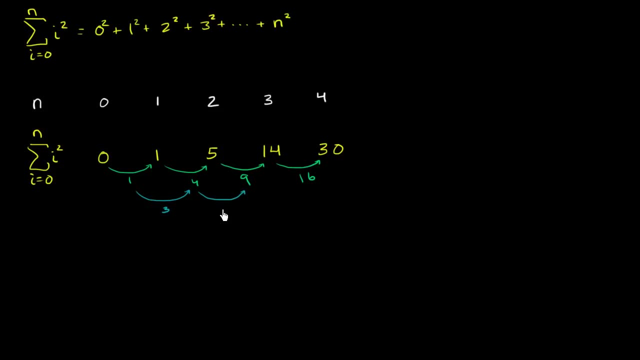 So the difference between those is 3.. Difference here is 5.. Difference here is 7.. So even the difference of the differences is increasing. But if this is a cubic function, then the differences of the difference of the difference should be constant. 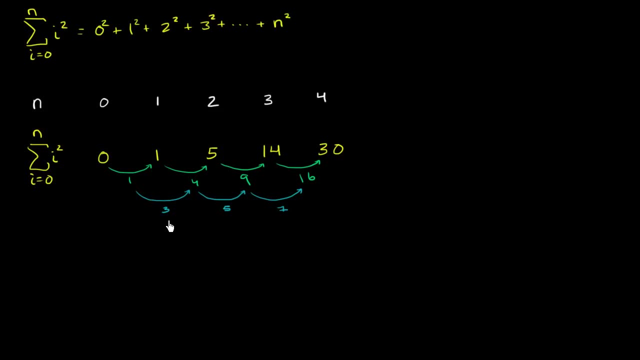 So let's see if that's the case, And you'll appreciate this even more when you start learning calculus. Let's see: the difference between 3 and 5 is 2.. The difference between 5 and 7 is 2.. 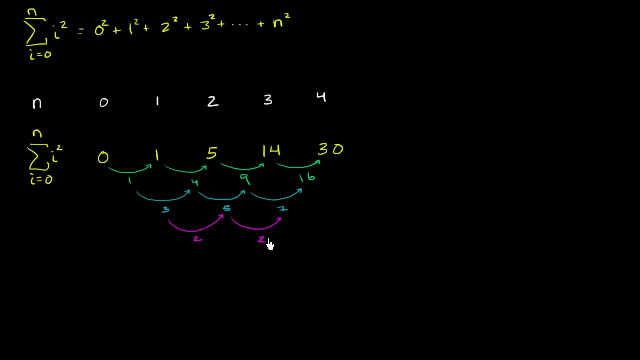 And so we keep having a constant shift of 2.. So the fact that the difference of the difference, of the difference, is fixed tells us that we should be able to express this as some type of a cubic function. So this we could write as this should: 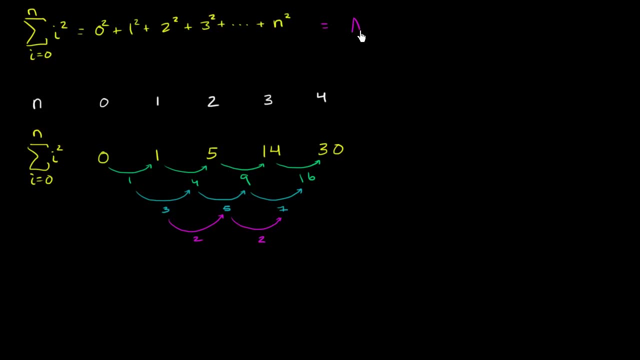 be equal to some function in terms of n And we could write it as a n to the third plus b, So that's n squared plus c times n plus d, And now we can just use what the inputs are, and the outputs are of these to solve for a, b, c and d. 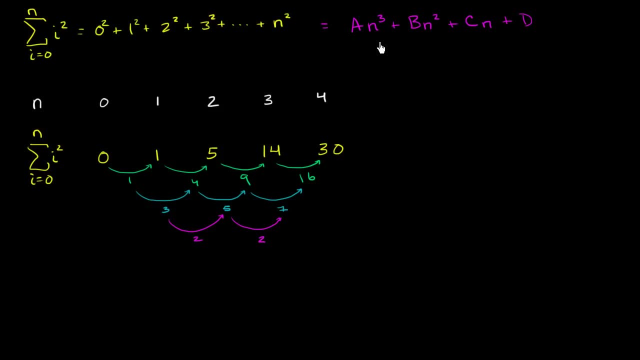 And I encourage you to do that. Well, let's first think about when n is equal to 0.. When n is equal to 0, this function evaluates to d. So this function evaluates to d, But that function needs to evaluate to 0.. 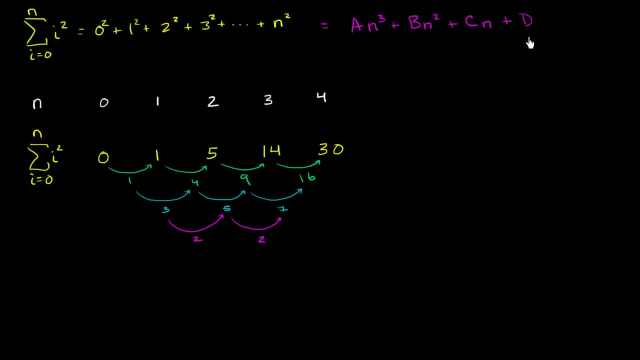 d needs to be 0.. So I'm just trying to fix these letters here to get the right outputs. So when n is 0, this expression evaluates to d And it needs to evaluate to 0. So d needs to be equal to 0. 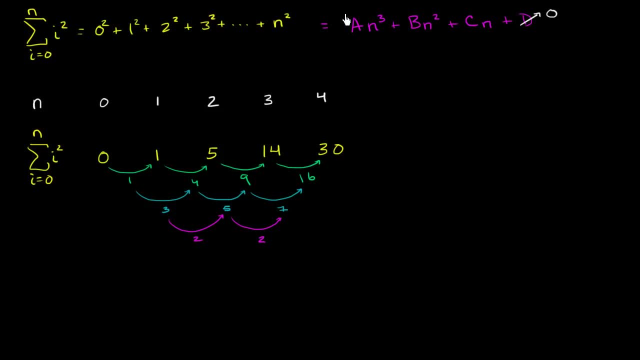 So d is equal to 0. Or we could just ignore it, So that helps us a little bit. We know from this data point we're able to whittle it down to it, having this form right over here, And so now we can take each of these inputs. 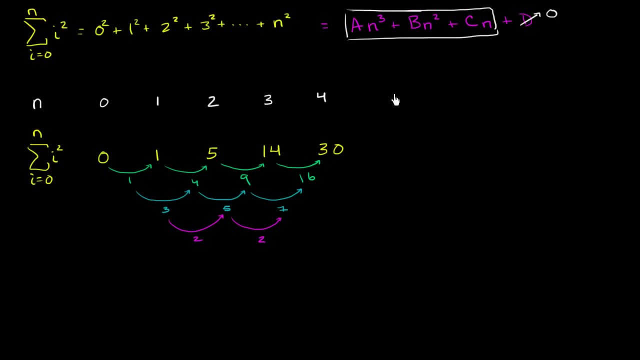 and figure out what their corresponding output is. So let's do that. I'll do that over here. So when n is 1, this thing evaluates to a times 1, to the 3rd power, which is just 1, plus b times 1 squared, which is just. 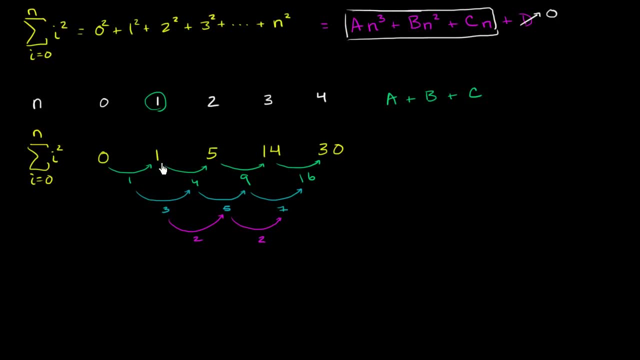 1, plus c times 1,, which is just c, And this needs to be equal to 1.. Now, When, When n is 2, we have a times n to the 3rd. So that's 8a plus 2. squared is 4, plus 4b plus 2c.